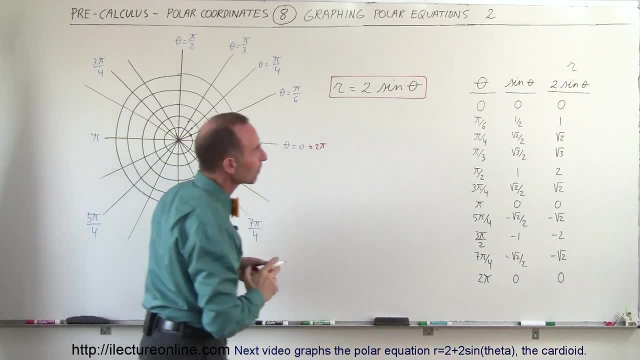 so at this point we're about right there. and then, finally, when theta is equal to pi divided by 2, the sine of theta is 1, and r is equal to 2, that places us right there. Okay, continuing on with that. now let's go a little bit faster. 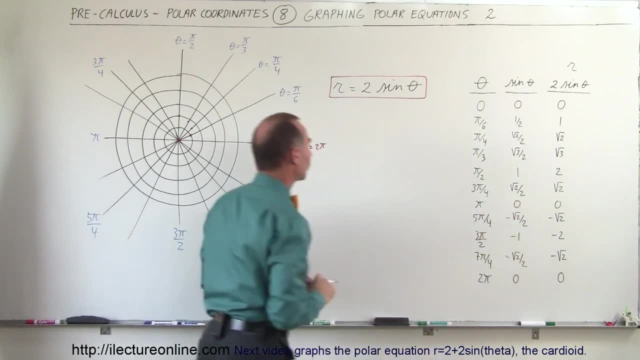 Now we go all the way to 3 pi divided by 2.. So 3 pi divided by 4, we have the square root of 2.. So 3 pi divided by 4, that would be this line. square root of 2 is right there. 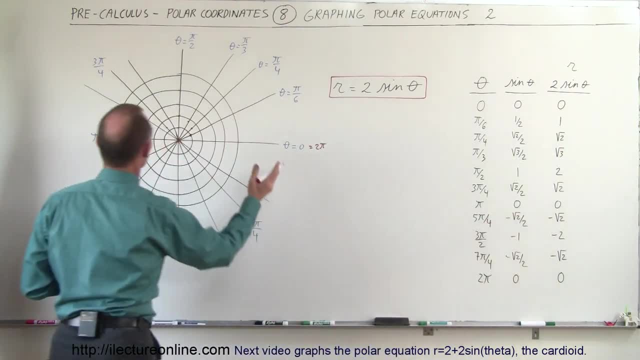 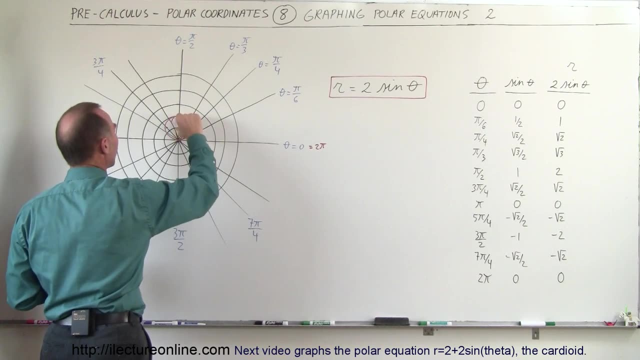 Then we continue on to pi, we get 0, so when we go all the way down to pi, we get back to 0. So then when we connect these dots, it looks like we have a little circle that has a radius of 1,. 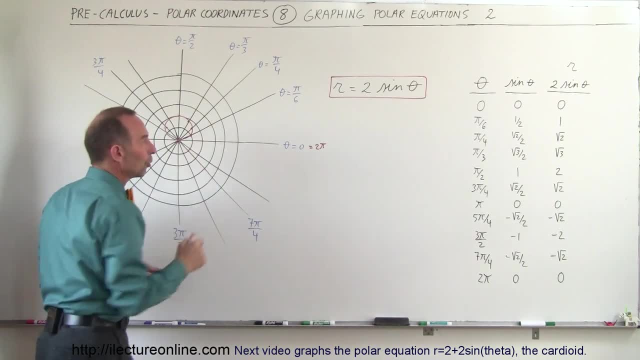 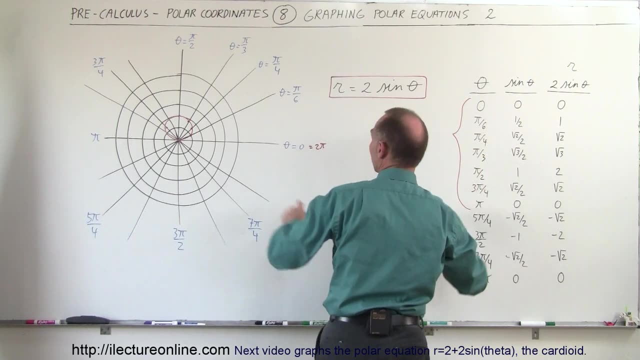 goes from r equals 0 to r equals 2, and that would be for the first set of numbers, from 0 all the way to pi. so that gives us this first circle. Now let me use a different color, so let's use purple. 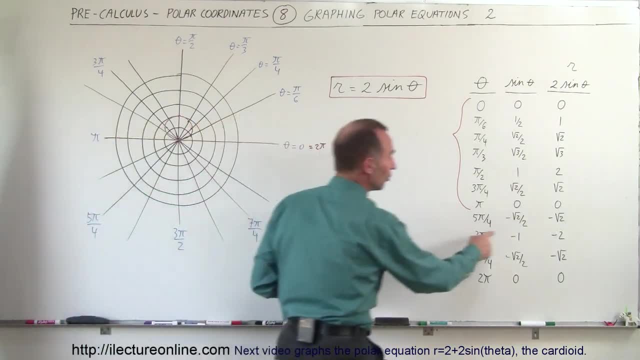 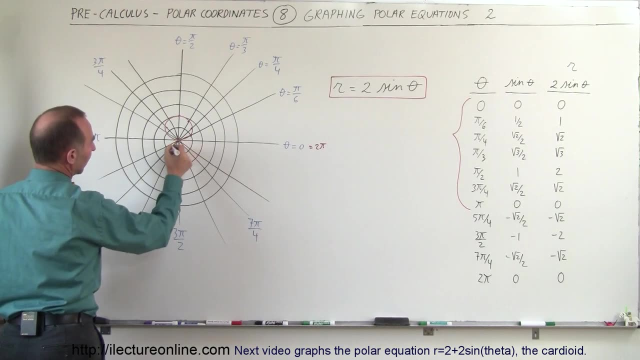 and now, if we continue to 5 pi divided by 4, notice now the number is minus the square root of 2, so when we go all the way to 5 pi divided by 4, right here. so instead of going out this direction, it's a negative number, so we should go back. 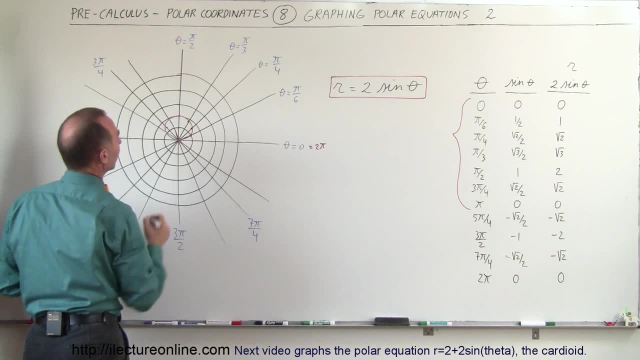 and how far back should we go to the square root of 2?? That puts us right back there again. so then we go to 3 pi divided by 2.. At 3 pi divided by 2, the number is negative 2, so when we are in this direction, it's negative 2,. 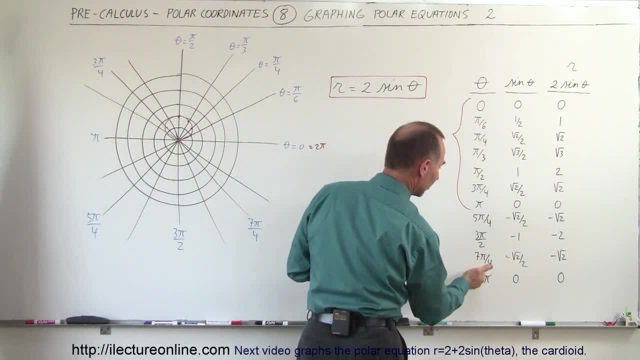 so we'll be back over here. then we come back to. let's see 7 pi divided by 4, the number is minus the square root of 2, so it's 7 pi divided by 4. when we are in this direction. 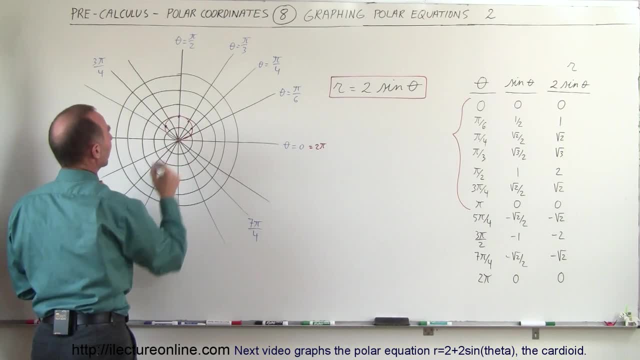 the number is negative, the square root of 2, that puts us right there. and finally, when we go all the way around to 2 pi, the distance is 0 again. so notice we come all the way around again and notice that when we have values, 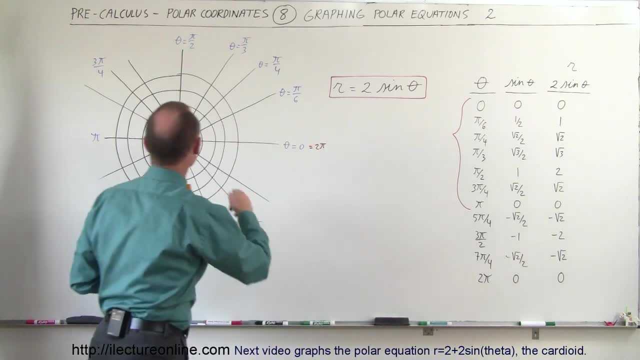 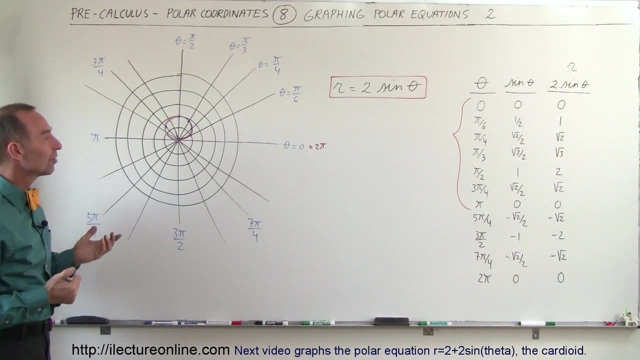 all the way from 0 to 2 pi. basically, we go around the circle twice and that would then be the graph of r equals 2 sine theta. so it's kind of interesting. so even though we go around it twice, we get the exact same coverage, the exact same circle. so we have a little circle of radius r.